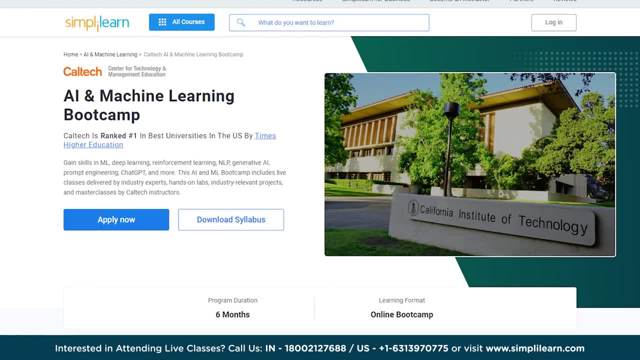 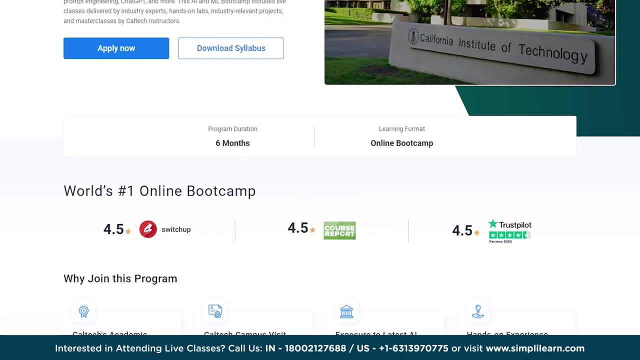 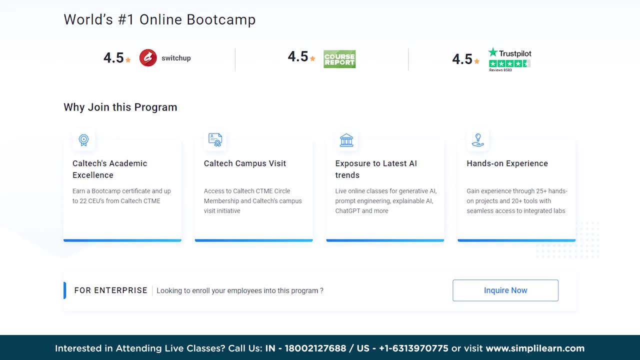 Caltech AI ML Bootcamp in partnership with IBM. This course covers everything from fundamentals to advanced techniques like machine learning, algorithm development and unsupervised learning. This AI and machine learning bootcamp in collaboration with Caltech will help you advance your career as an AI ML specialist. The AI ML bootcamp. 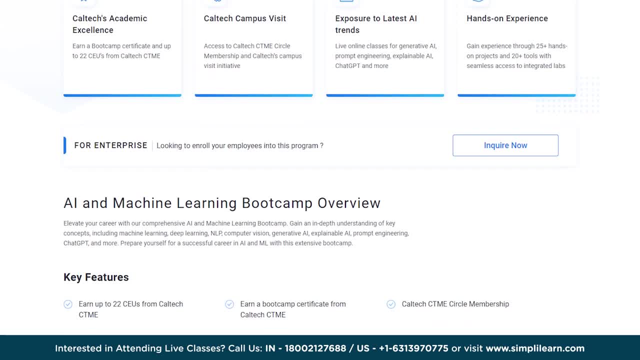 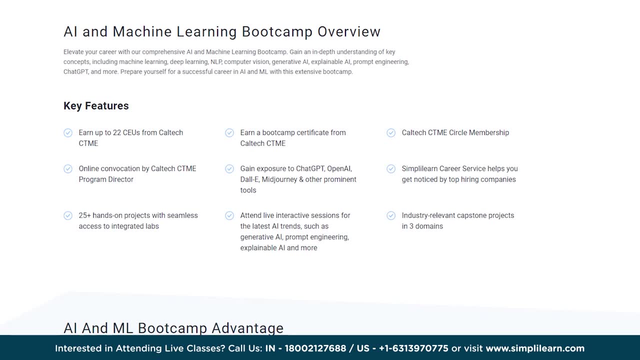 includes the live classes delivered by industry experts, hands-on industry relevant projects and master classes by Caltech professors. Key features of this amazing machine learning course include 22 SEEDS from Caltech CTME Online Convocation by Caltech CTME Program Director. 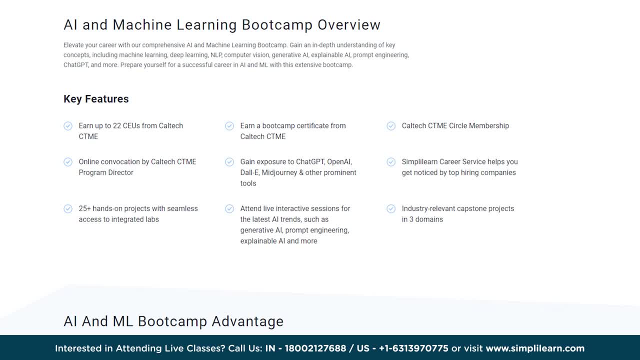 Simply Learn. Career Service helps you to get noticed by top hiring companies. Earn a Bootcamp Certificate from Caltech CTME Industry-Relevant capstone projects in three domains: Caltech CTME Circle Membership 25, plus hands-on projects across industry verticals and integrated labs. 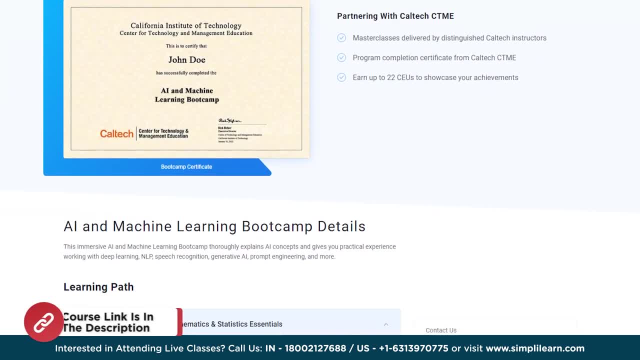 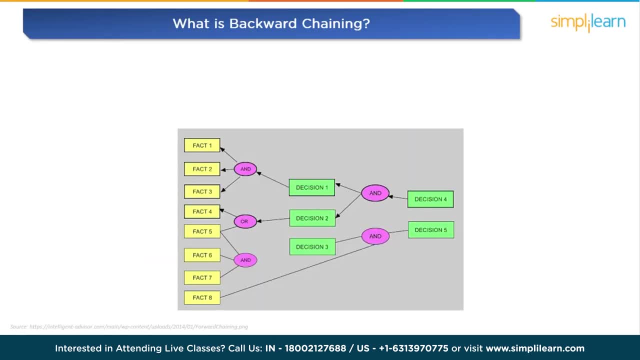 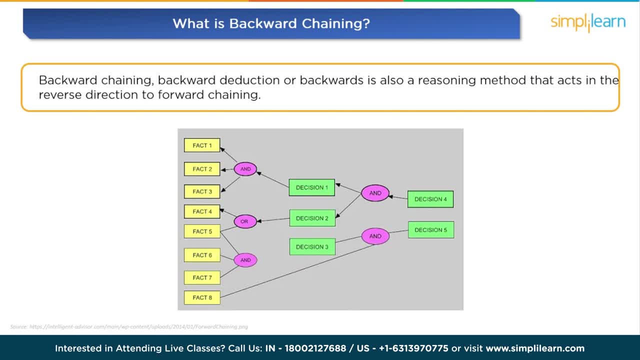 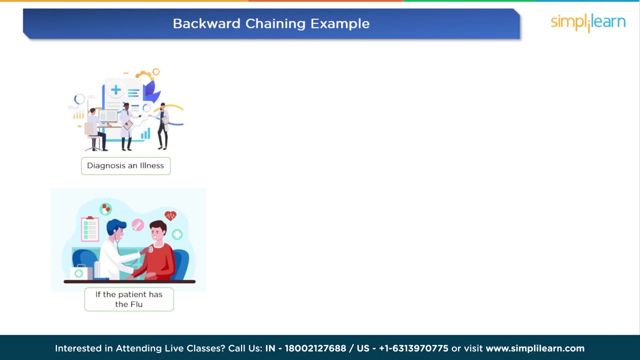 the top-down approach involves using decision or goals to reach the facts. the backward chaining is the backtracking process of finding usage in diagnostic debugging and prescription. here is a simple real world example of backward chaining scenario: diagnosing an illness. here we have a goal to determine if a patient has a flu, rules and facts if a patient has a fever. and 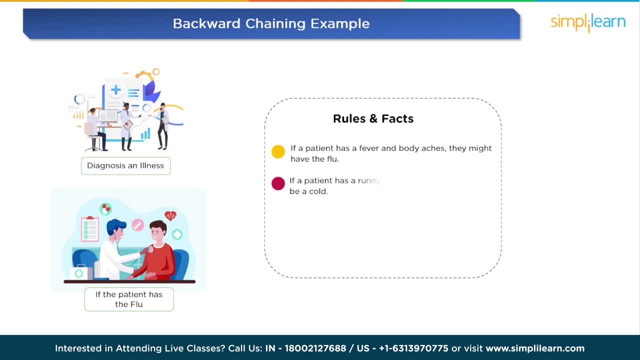 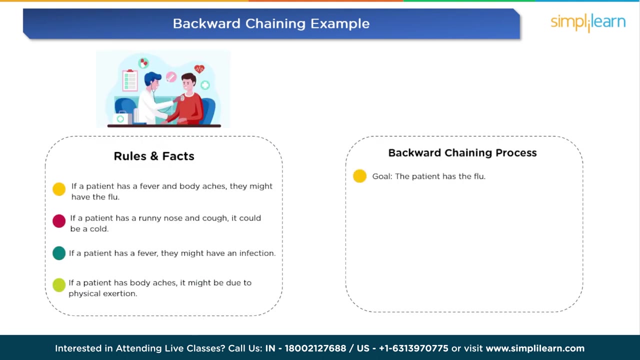 body aches, they might have the flu. if a patient has a runny nose and cough, it could be a cold. if a patient has a fever, they might have infection. if a patient has body aches, it might be due to physical exertion. in this example, let's say we start with the goal of determining if a patient 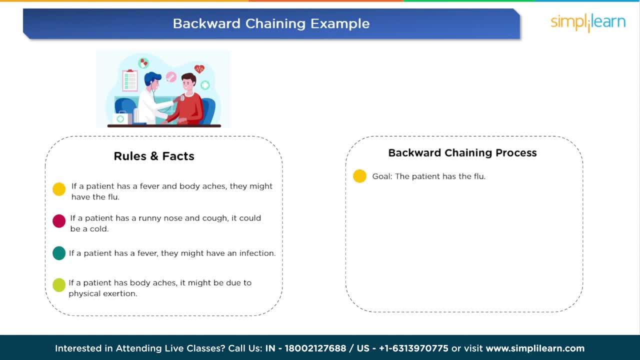 has a flu you. so how does a backward chaining process works? look at rule one: the patient has a fever and body aches. at rule three, the patient has fever. look at rule two: the patient has runny nose and cough. this rule doesn't apply. look at rule four: the patient has body aches based on the backward. 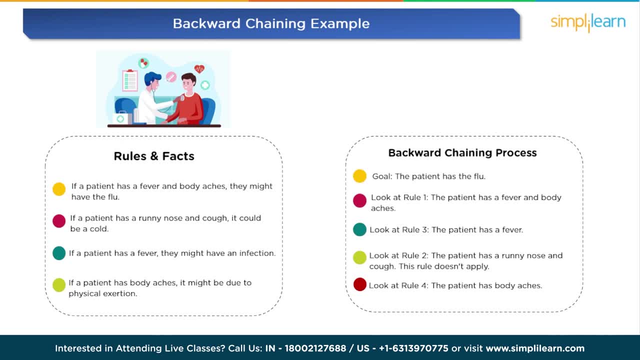 chaining process, the evidence suggests that patient might have the flu because of a fever and body aches. this is the chain of reasoning that leads to the conclusion that patient could have flu. in essence, backward chaining starts with the desired outcome and traces the path backward through rules and facts to find supporting. 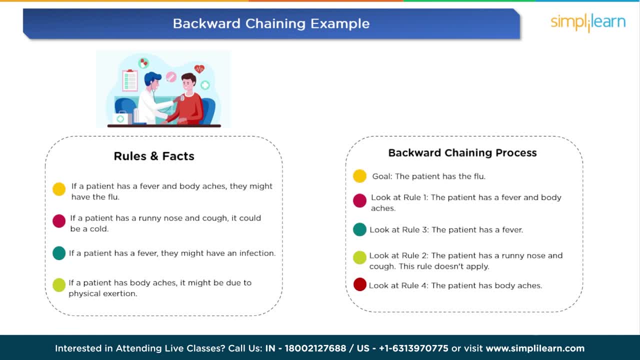 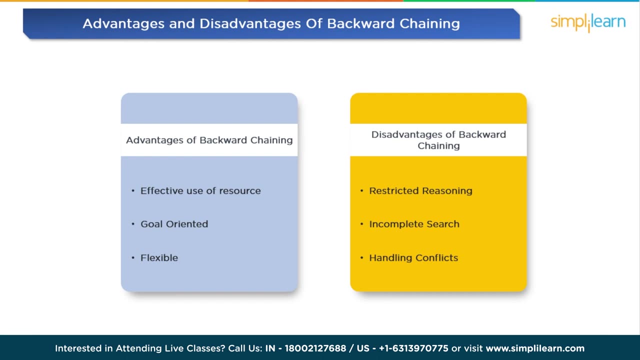 evidence. it's commonly used in diagnostic systems, troubleshooting and other scenarios where the goal is to determine the causes or conditions that lead to a specific result. moving to the advantages and disadvantages of backward chaining. advantages of backward chaining: backward chaining offers optimal resource usage by efficiently concentrating on essential laws or requirements for goal. 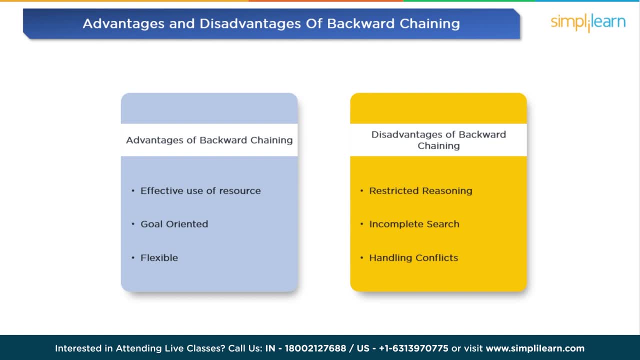 achievement, resulting in time and computational savings. it's goal oriented, commencing from predefined objectives and tracing back to identify relevant supporting situations or rules. additionally, its adaptability allows easy customization across various applications, showcasing a broad range of problem solving capabilities. disadvantages of backward chaining: while employing backward chaining for problem solving, it functions unidirectionally. potentially. 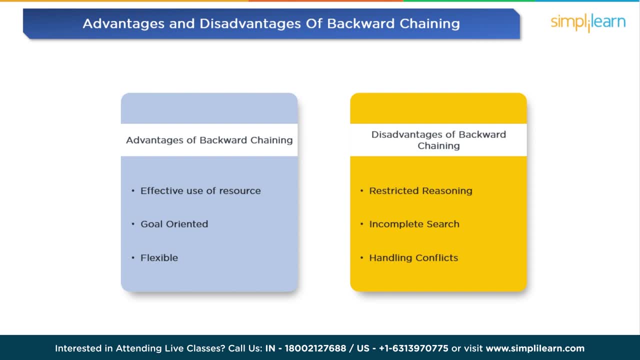 lacking the ability to generate innovative solutions or insights not explicitly programmed. there are instances of limited exploration where it may yield incomplete outcomes and overlook comprehensive solution exploration. additionally, conflict resolution can be challenging with backward chaining, especially when reconciling discrepancies or clashes among various laws or facts. let's move to forward chaining. forward chaining, forward deduction or forward reasoning is a 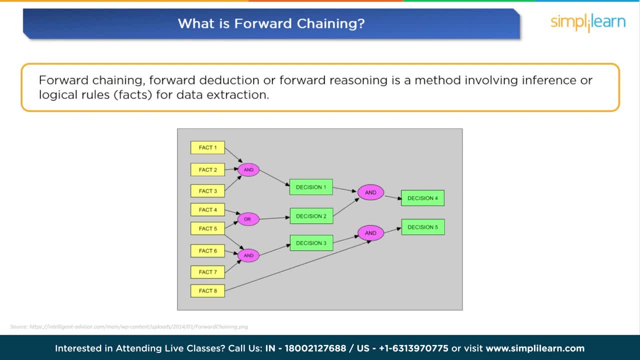 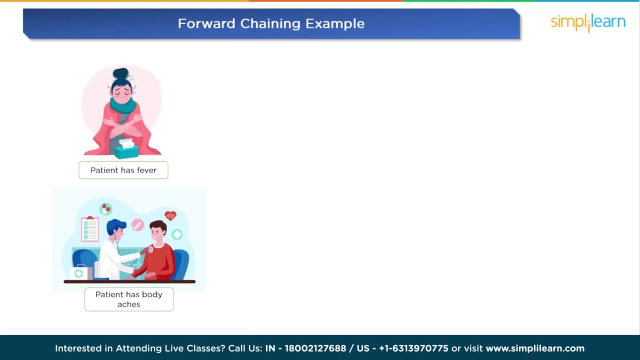 method involving inference or logical rules, facts for data extraction. it is a bottom-up approach performed redundantly to reach the endpoint or goals. it begins with evaluating existing information, followed by manipulation based on the knowledge base. existing information can be as facts, derivations and conditions. let's move to a real-world example of forward chaining. 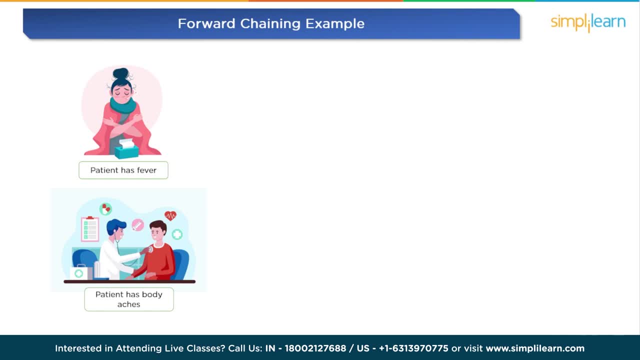 here we have a scenario of diagnosing an illness. we will consider following facts: patient has a fever and patient has body aches. so let's look at the rules. if a patient has a fever and body aches, they might have flu. if a patient has a runny nose and 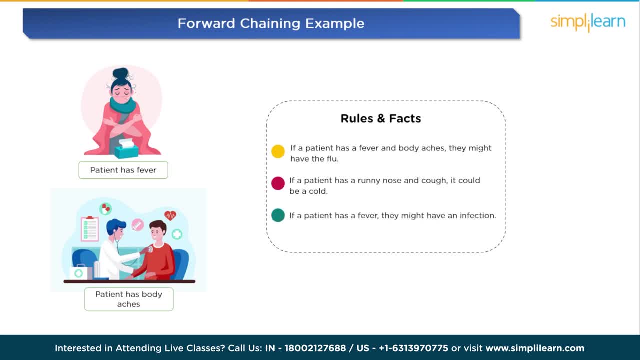 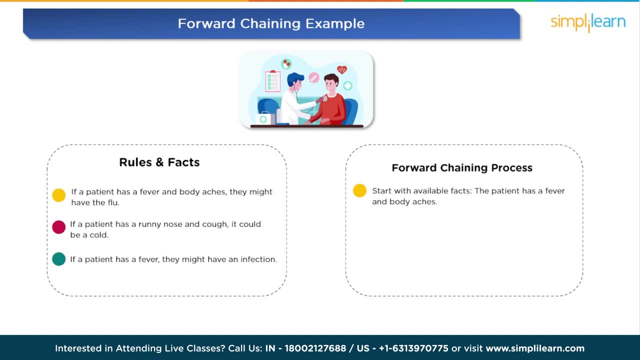 cough, it could be a cold. if a patient has a fever, they might have infection. so how does this forward works? Start with the available facts. The patient has a fever and body aches. Apply rule 1. The patient has a fever and body aches suggesting they might have flu. This conclusion might have 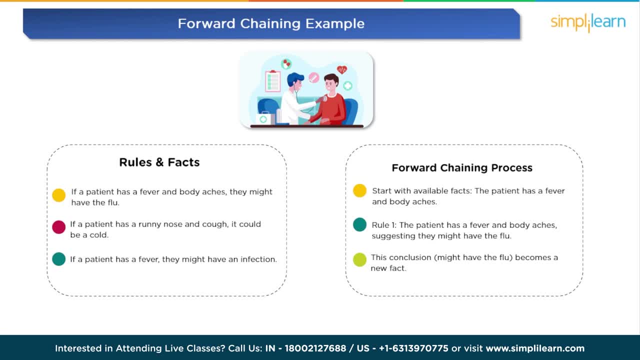 the flu becomes a new fact. At this point, forward chaining process has derived a new conclusion based on the available facts and the rules. The process could continue with additional rules and facts to derive further conclusions. In a sense, forward chaining begins with the known facts. 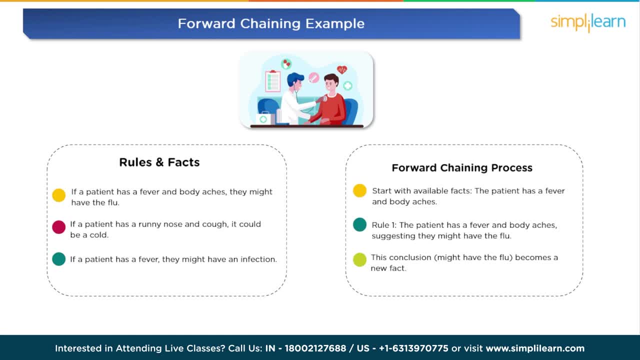 and applies rules to generate new information or conclusions. It's often used in systems where initial data is available and the goal is to deduce new information or outcomes based on the data and predefined rules. So what are the advantages and disadvantages of forward chaining? 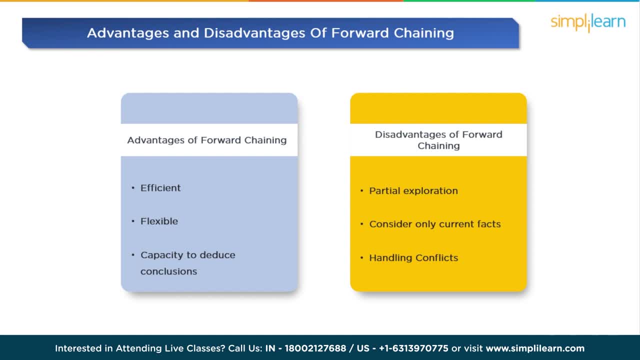 Advantages of forward chaining. Forward chaining demonstrates its efficiency by leveraging existing findings. It is not a system of data collection. It is not a system of data collection. It is not facts or conditions to achieve solutions potentially resulting in time and computational resource preservation compared to alternative methods. Its flexibility shines through its 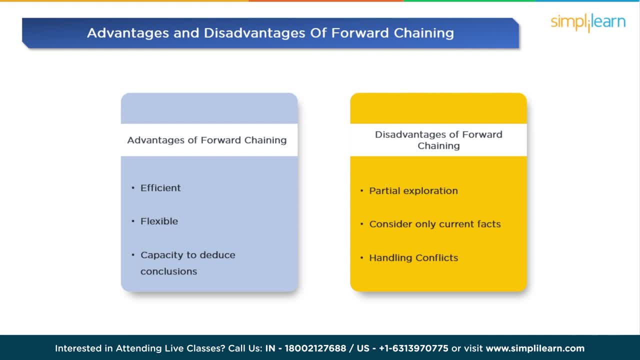 adeptness at tackling various problem types and its simplicity of adaptation for differing goals. Furthermore, due to its capacity to swiftly deduce conclusions from a given set of facts or conditions, forward chaining is particularly suitable for real-time decision-making situations. However, it's important to consider the potential disadvantage of forward chaining. 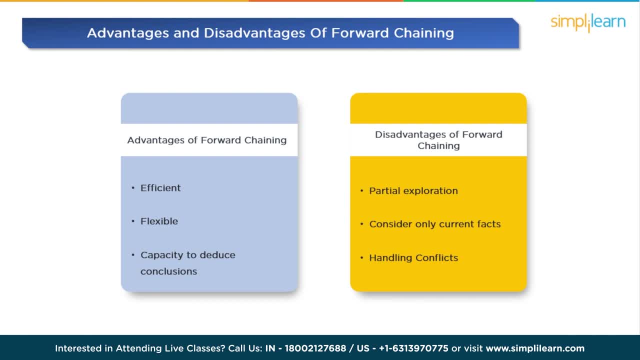 So here are a few disadvantages of forward chaining. Forward chaining may exhibit partial exploration, leaving some potential solutions inadequately explored or generating incomplete results. The method's limitation is considering only current facts or conditions might result in an absence of a global perspective, potentially leading to inaccurate conclusions due to a lack. 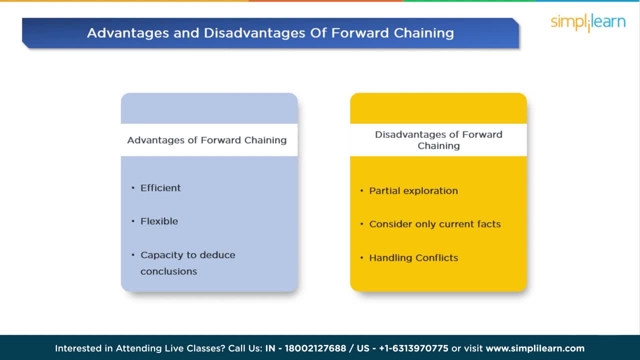 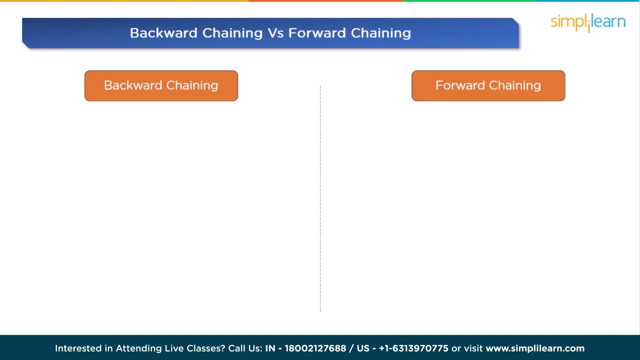 of broader contextual understanding. Furthermore, handling conflicts within forward chaining, especially when faced with inconsistencies or clashes among multiple facts or rules, can prove to be challenging. Now let's see the major difference between backward chaining versus forward chaining. Backward chaining and forward chaining are two distinct inferences techniques used in. 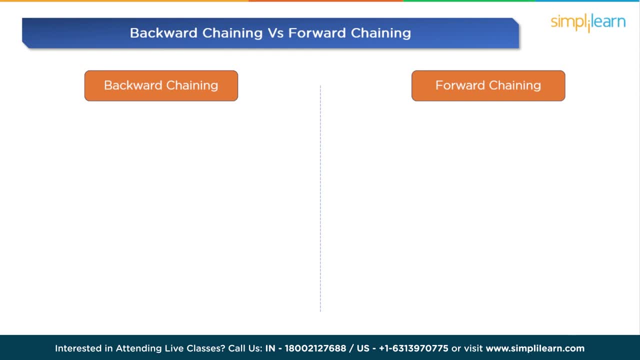 artificial intelligence and expert systems for problem solving and reasoning. They differ in their approaches and how they derive conclusions and available information. Here's a comparison between two: Backward chaining starts with a specific goal or conclusion and works backward through a set of rules and facts to find evidence or conditions that supports the goal. 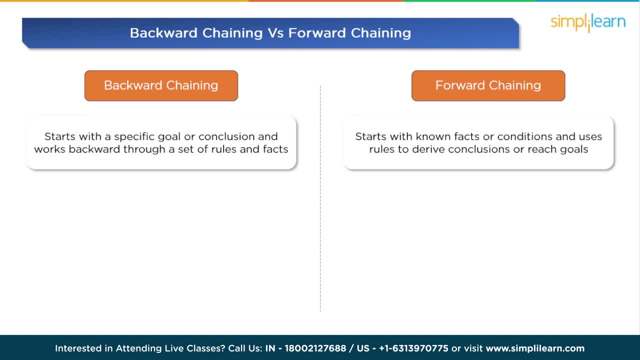 Forward chaining starts with known facts or conditions and uses rules to derive conclusions or reach goals. It iteratively applies rules to known facts to generate new information. Backward chaining is commonly used in diagnostic systems, troubleshooting and scenarios where the goal is to determine how the outcome of the decision is going to be achieved. The 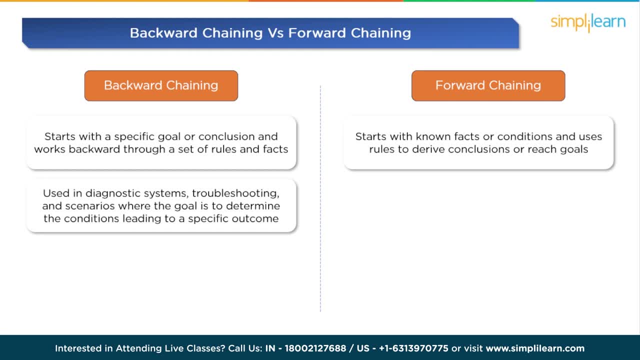 the causes or conditions leading to a specific outcome. Forward chaining is often used when the initial data is available and aims to reduce new information or outcomes based on that data and predefined rules. Backward chaining can be efficient when goals is known and the system seeks to establish the reasons behind goal. Forward chaining can be efficient when the 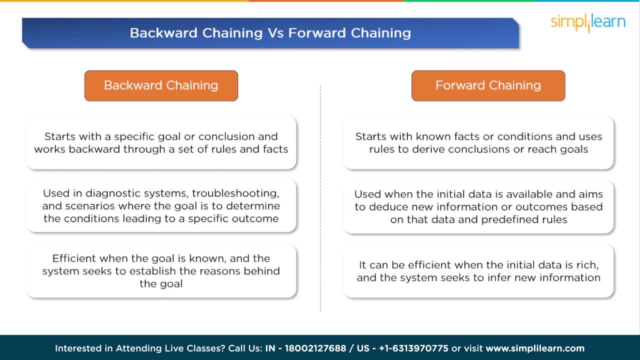 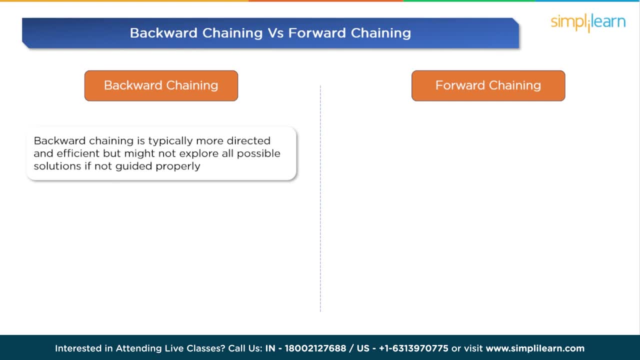 initial data is rich and system seeks to infer new information. Backward chaining is typically more directed and efficient but might not explore all the possible solutions if not guided properly. Chaining explores new conclusions as they have become available, potentially exploring a broader range of solution, but it might not be directed if not properly guided. And with that we have come to. 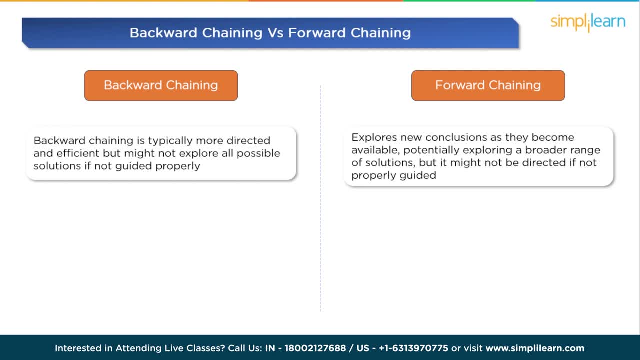 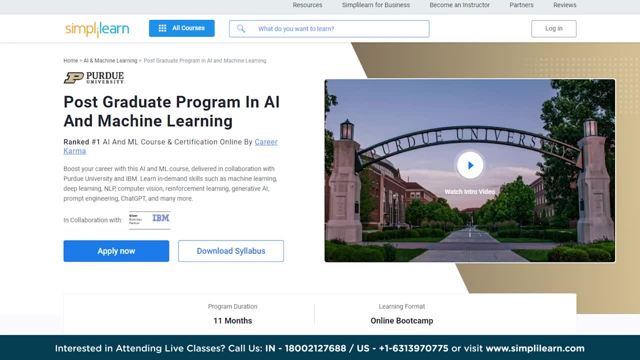 the end of this video on backward versus forward chaining. I hope you have find this information valuable. Do check our postgraduate program in AI and ML in partnership with Purdue University and Collaboration With IBM to upskill yourself in thrilling field of machine learning. don't forget to check the 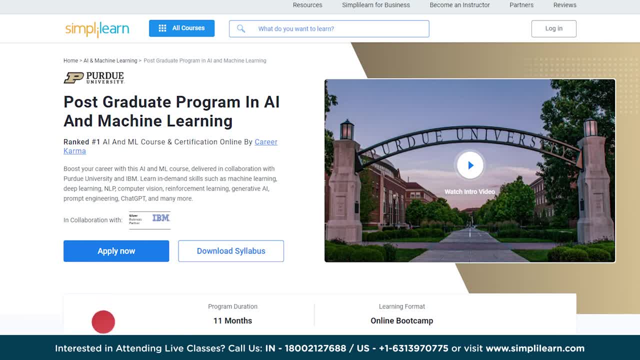 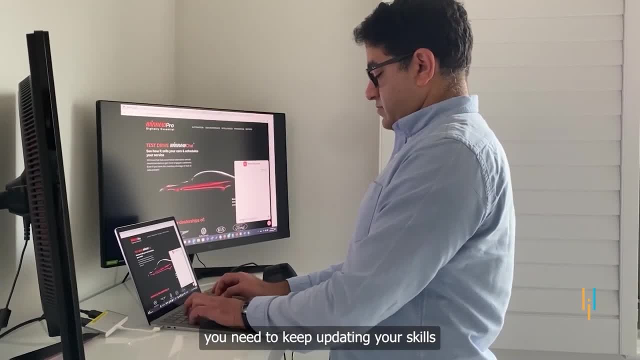 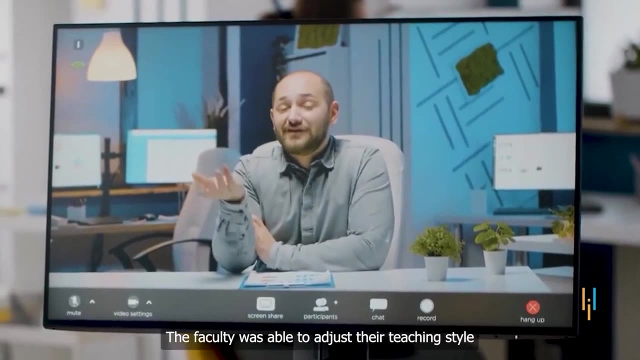 course link in the description box. Let's take a minute to hear from our learners who have experienced huge success in their career. You need to keep updating your skills. The course material was comprehensive and the faculty was extremely experienced. The faculty was able to. 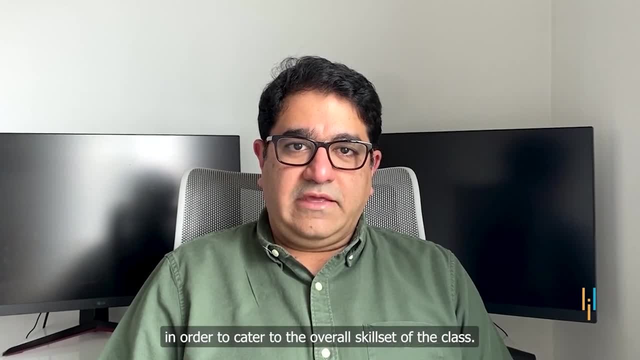 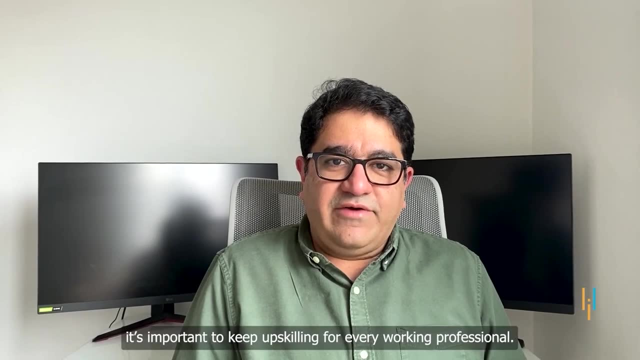 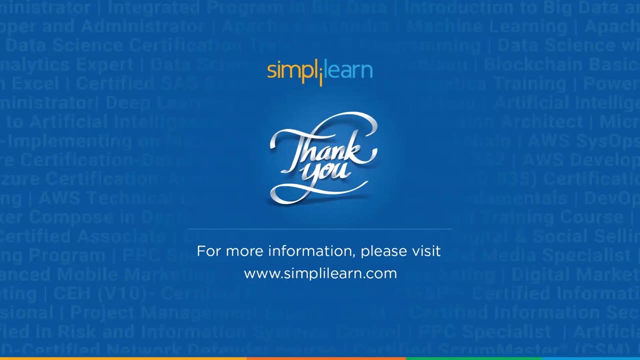 adjust their teaching style in order to cater to the overall skill set of the class. In the rapidly changing world of technology, it's important to keep upskilling for every working professional. Stay relevant, continue learning. Please ask any questions about the topic covered in this video.